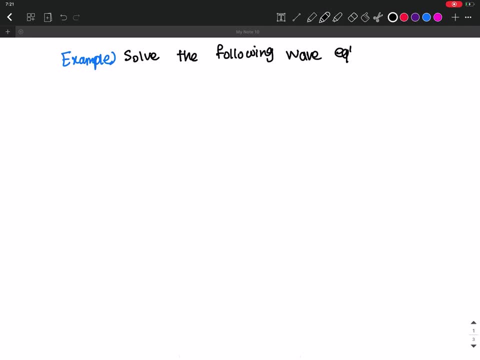 wave equation. so the equation that is given here is: partial square U over partial T squared equals to C square. partial square U over partial X square for x between 0 and L. and the boundary conditions that are given here are: I, Director del squared, меня here are: u at zero, at x equals to zero at any time is always zero. so at the 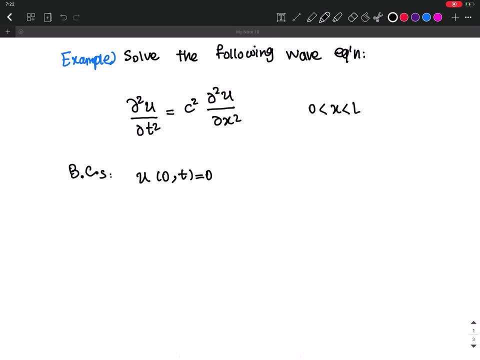 left boundary is always zero and this means that, for example, if this is a wave, we have a fixed end because the displaced- if you think of this, of you, as displacement. so this means that we have a fixed end and we have a zero displacement, right, because the displacement at the left boundary should. 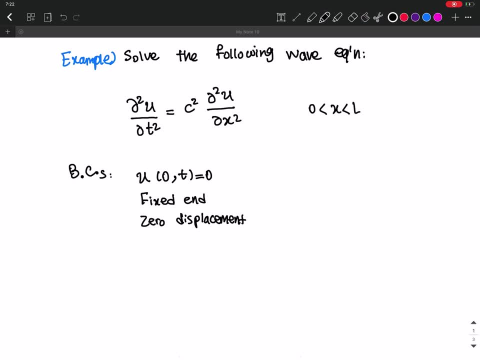 be zero, and the second boundary condition that is given is: x equals to zero, and the second boundary condition that is given in this problem is u, the first derivative of u with respect to x. at L, so and T is 0, so at the second, the right boundary. so if you remember what is this, 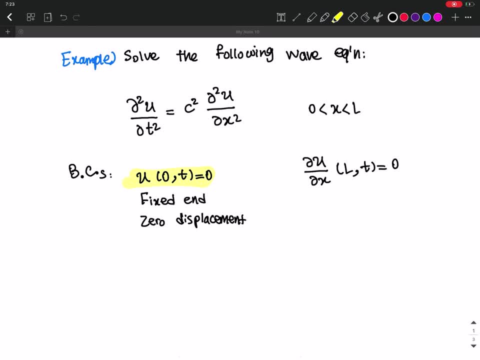 band. what is this boundary condition? the type of this, if you remember, this is directly boundary condition that we talked about and this one is Newman right- where we get, where we specify the derivative of the solution at a specified point- okay, specific point- and this boundary condition states that. 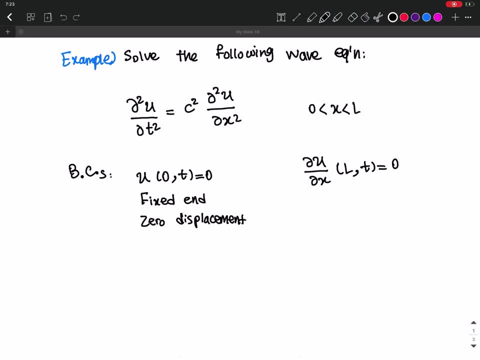 the derivative of you. if you is like displacement at X, at L, X equals L- should be zero and this means that we have a free end. so it can run, it can go up and down, right, so it can be. it can say: if you have like a beam, it can go up down, it can do all the things right, go. 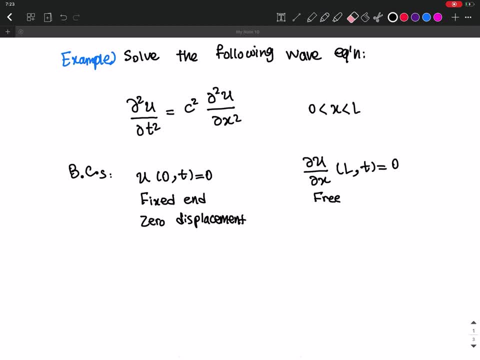 up down. so we have a free end. it's not like this one that it should be fixed to somewhere. so we have a free end. and at the right, at X equals to L, and but the thing is we have a zero strain and stress boundary condition. right, because your stress, if this is strain, if your displacement is, 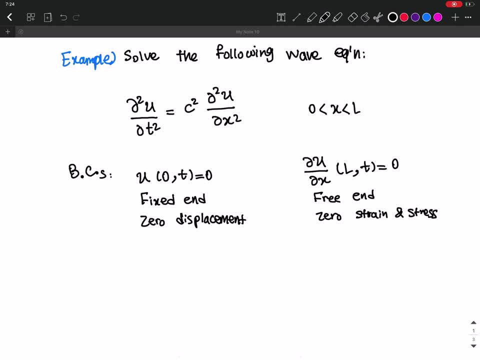 zero is gonna be zero, so this is what we call like strain or stress for people who are familiar with mechanics. okay, so this is the boundary condition and the initial. we also need initial condition for this problem. so the initial condition of this problem is U at X and 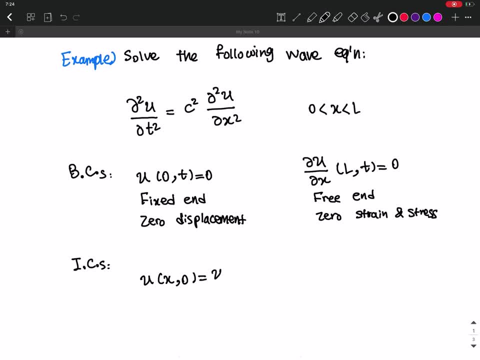 zero is a function of zero which we call U, not X at T equals to zero. and then we, we are, we need another boundary condition, initial condition, and our so d, partial u or partial over partial t at x and t equals to 0, is function which we call. 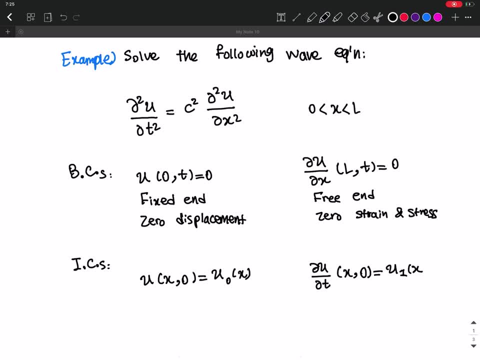 as given function of what you call u1 x. okay, so this is a problem statement and we want to solve this. pde, p, given these boundary conditions and initial conditions. okay, and this is, as you remember, this is the equation for wave, a wave equation, and you know the characteristics. how does this look like? and now we want to solve this with the. 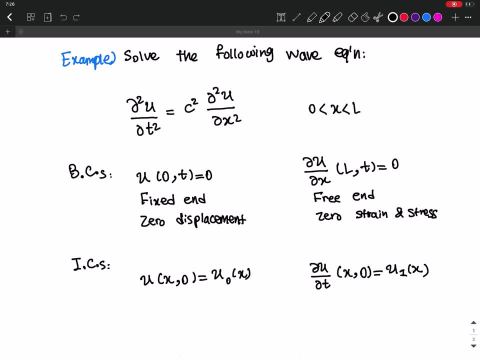 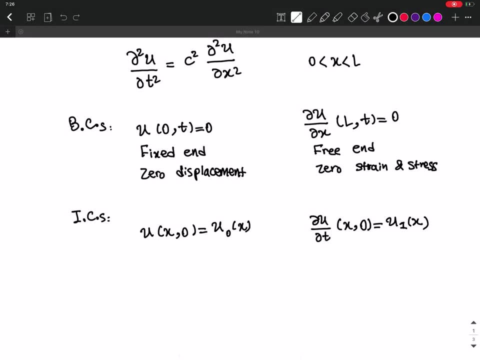 help of a separation of variable technique. before i go further, i just want to give you a physical intuition of uh. how does this uh problem look like? actually, if you know, you want to know the basic physics and gain some insights, so i can just plot these boundary conditions and just show you what do they mean. 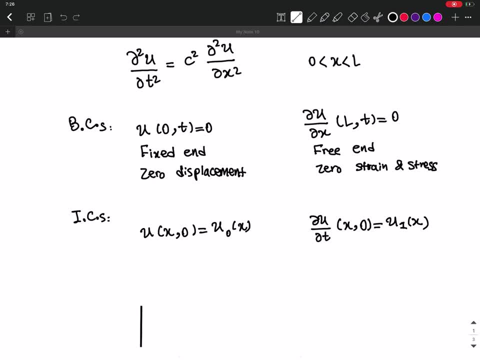 so say again, if you have similar to the previous part which i showed for a heat equation, so say: now you have a beam, so let me just draw it a beam, okay. so this is zero at x equals to zero, and this one is x, and this is at x equals to l. so the the first, uh, so the first boundary at the left means that 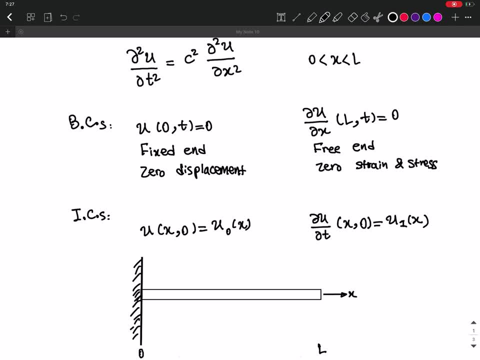 we have a fixed end, right. so this uh end, as you see, is fixed here and on the right, the right boundary, based on this equation, which is about the imposed boundary condition, we have a free end. this means that this is fixed: beam can go up and down, can go up or down, right, and can oscillate, can vibrate. 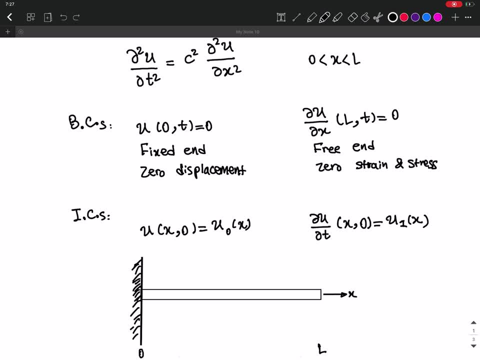 okay, and so the question is, what we want to find is, for example, here this is gonna, this can vibrate like this, or this can vibrate like this, right? so these are different modes of vibrations for this beam, right? so this can go up like this or can go down, and we want to find these modes of vibration for this, for this. 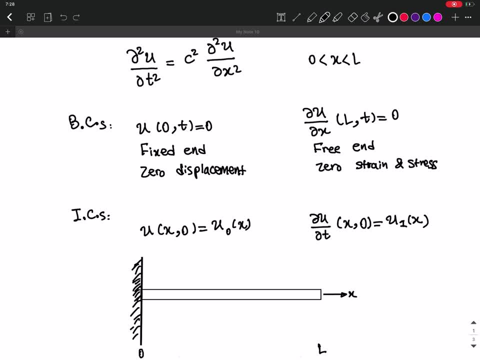 problem, right? so for this beam, for example, and the governing equation here is this wave equation, and so these are the boundary conditions which are similar to this, and the only thing here is we have the initial condition, so we know the initial condition. you, at time 0, what is? 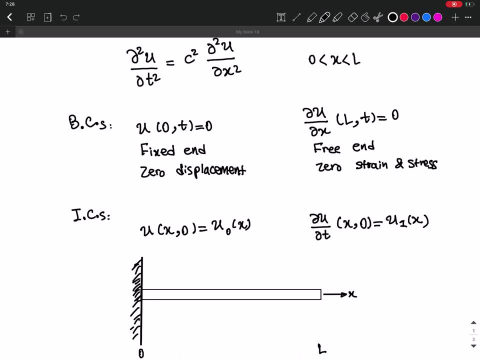 that we know that displacement, for example the initial displacement, could be something like this: and this is like u 0- X, and also we know the DAVID positive of that too. so we know the derivative of the ~~~. initial displacement for the atomic was 0. at how it's gonna go propagate in time. 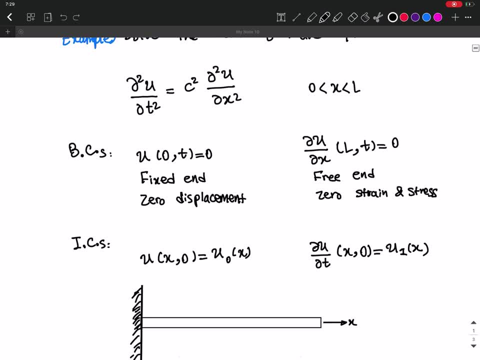 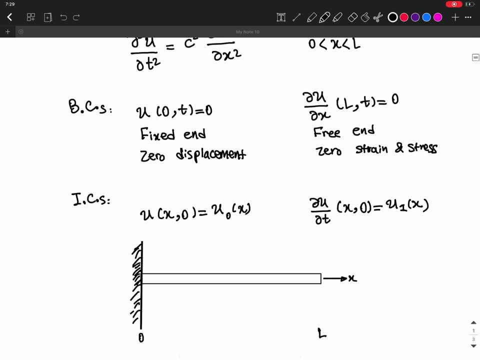 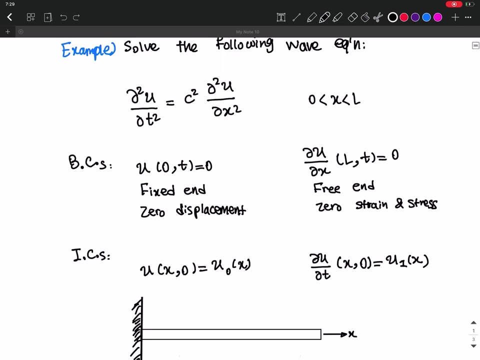 okay, so you had had. this is kind of the problems statement. I gave you the formula that you want to solve the PDE and also give you some physical intuition that how does this problem look like and what we want to do next is to solve these PDE given these boundary conditions, initial conditions we see. 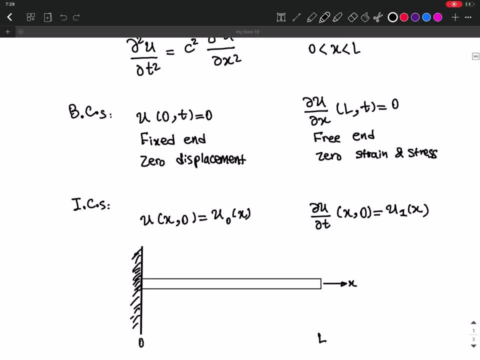 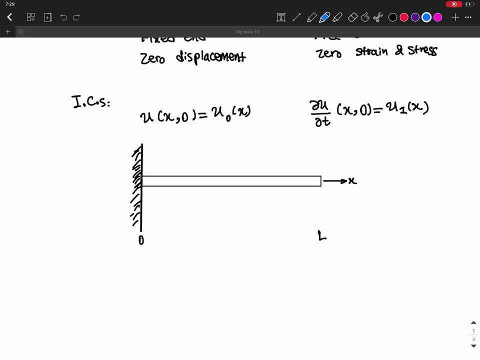 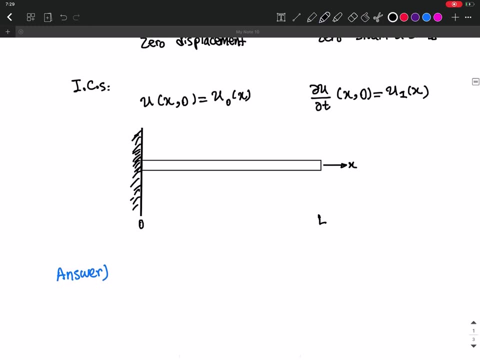 help of separation of variable technique. okay, so let's get it started and I'm gonna write answer for this example. so the first thing I'm gonna do in the separation of variables, I'm gonna propose a solution and separate the variables. so I separate X and T, which is space on time variables here, so separate. 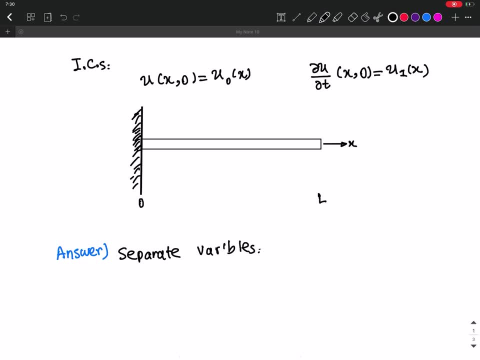 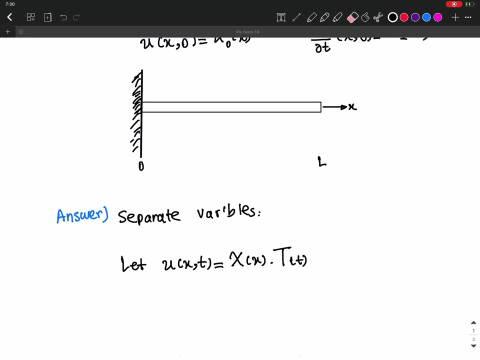 variables. so let's U X, U X and T B. so we propose this solution: a function of X, X capital X, multiplied by T capital T, which is a function of time, right? so we separate these two variables and then we we let this UP to be this function and then I'm gonna calculate, substitute this into the. 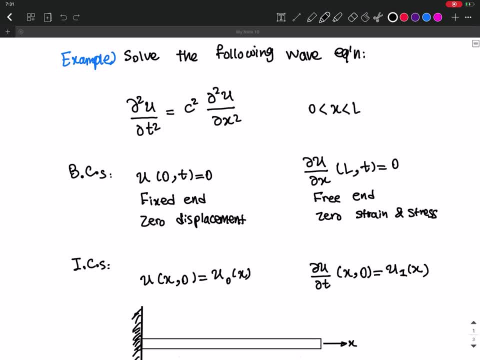 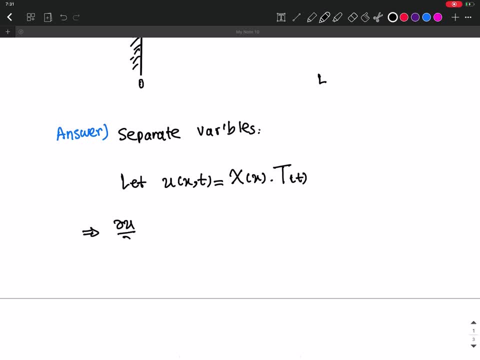 original PDE that I have here. okay, so I need to calculate the terms. so the first term is partial U over partial T. let's calculate what it is it's going to be. X is not a function of time, so I just write: it is late, that's. it acts like a. 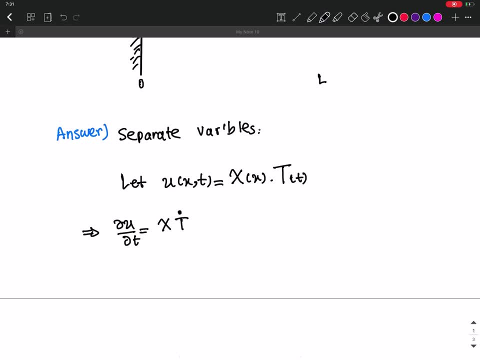 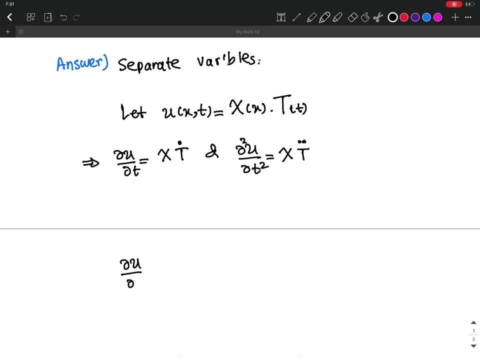 constant here times t dot. and the second derivative of u with respect to time is simply x, t double prime right, Because x, again is a constant here. Similarly I do it for x and take the derivative with respect to x. So partial u over partial x is going to be x dot time t. Again, t acts like 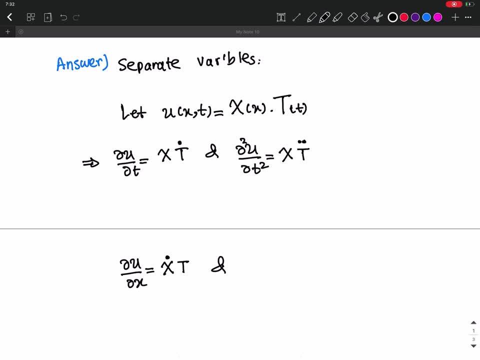 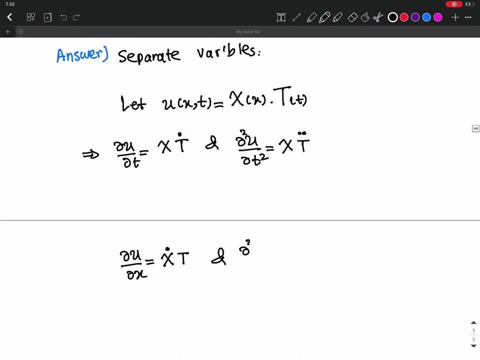 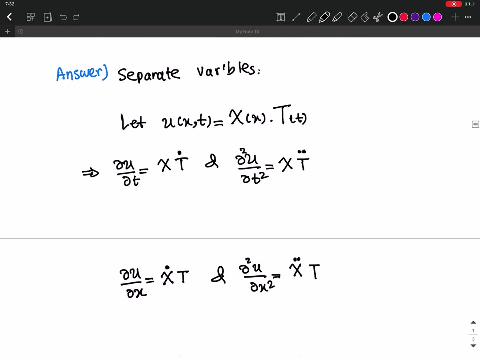 a constant here, because it's not a function of x. And then the partial square u over partial x square is x double dot times t. okay, So if u is this, these are going to be the derivatives of that function. okay, So now we substitute these into the wave. 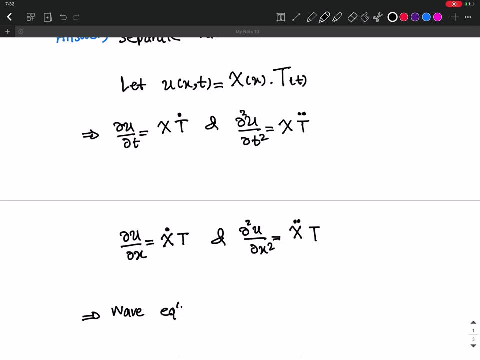 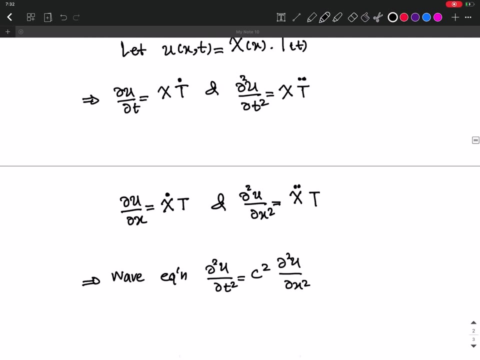 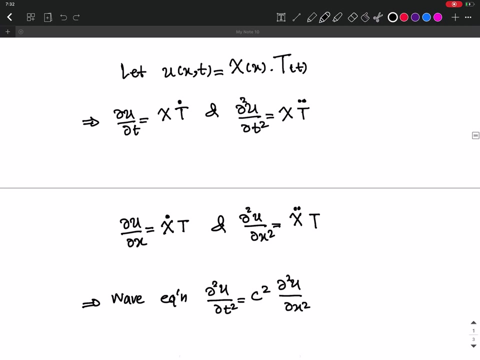 equation that we had. So the wave equation that we had was: partial u, u, partial square u. partial t square equals to c square. partial square u over partial x square. okay, so i just write this down. i have this and this and this is going to give me. 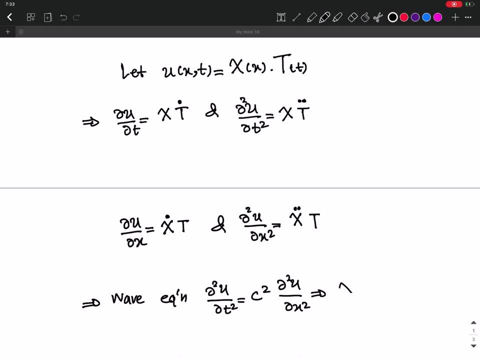 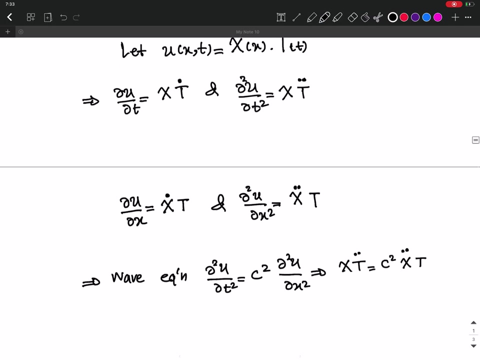 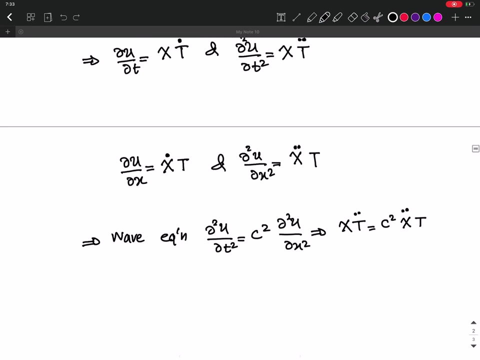 this equation: x, t double prime equals to c square x, x double prime, t. right, if you just substitute this, these definitions that we had, into the wave equation, we are going to get this equation and then we use the technique we uh previously used for the last problem that we solved and we separate the. 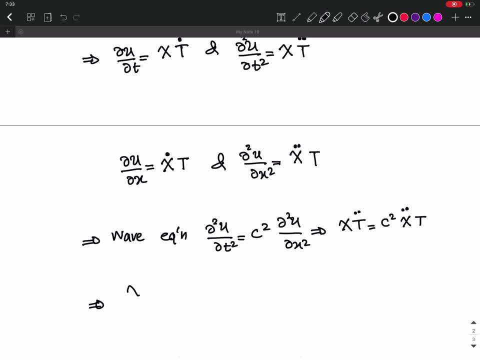 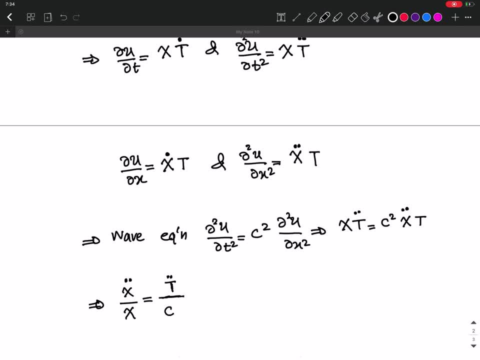 over t c square t. over t c square t. right c square t. this is uh, i find it from this equation. this is uh, i find it from this equation. this is uh, i find it from this equation, and uh, as you remember, because these are, and uh, as you remember, because these are. 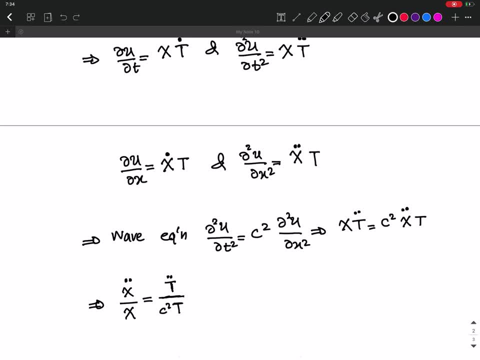 and uh, as you remember, because these are two functions, two functions, two functions of x and time, so two different variables of x and time. so two different variables of x and time, so two different variables. so this can be a function of, so this can be a function of. 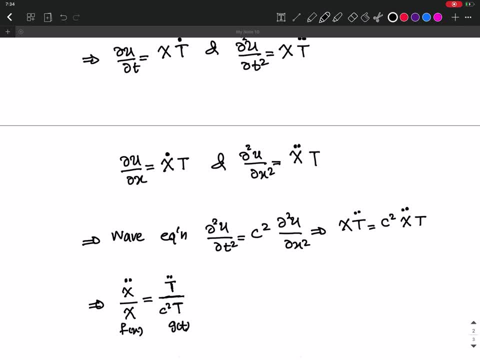 so this can be a function of x and this can be a function of time x and this can be a function of time x and this can be a function of time. so, the only way that they can be so, the only way that they can be so, the only way that they can be equal, 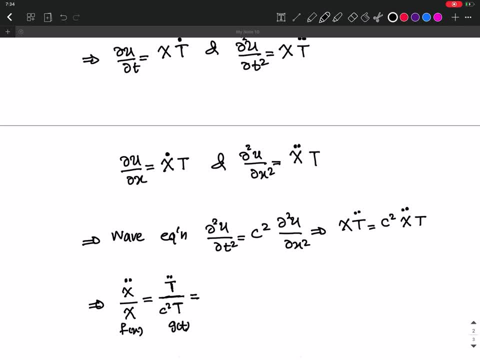 equal equal to each other is if they equal to a to each other, is if they equal to a to each other, is if they equal to a constant, constant, constant. and i write that constant as minus and i write that constant as minus and i write that constant as minus. lambda square. 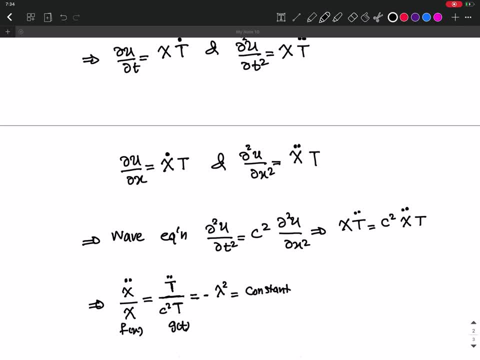 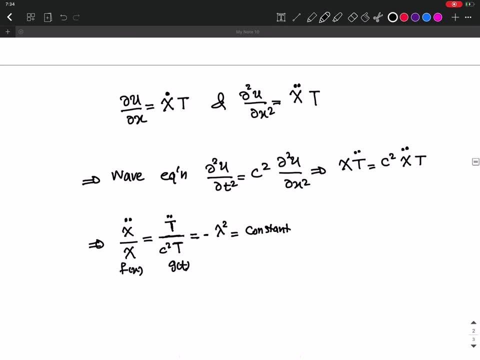 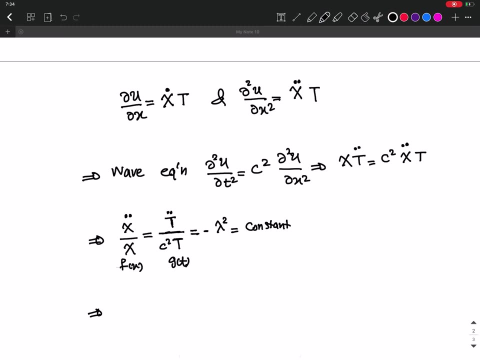 lambda square, lambda square. so this is a constant, and so i can, and so i can, and so i can. i will get two sets of equations. i will get two sets of equations. i will get two sets of equations. the first set of equation is gonna give. the first set of equation is gonna give. 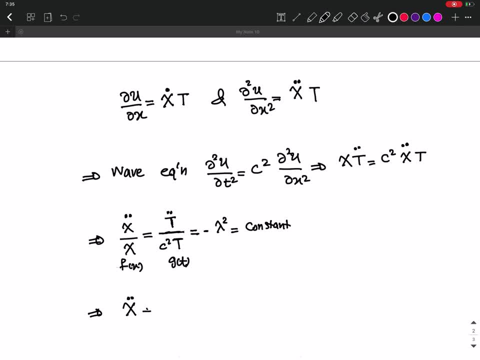 the first set of equation is gonna give me me me x, double dot plus lambda square x, x, double dot plus lambda square x, x, double dot plus lambda square x equals to zero, equals to zero, equals to zero. and the second set is going to be: and the second set is going to be. 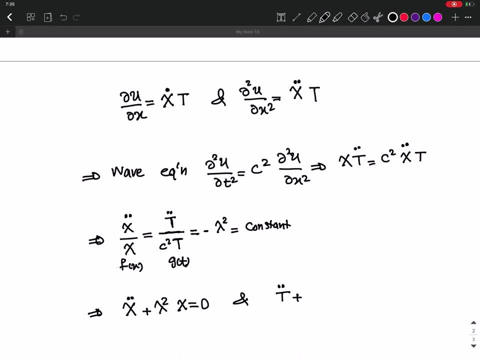 and the second set is going to be t double dot plus t, double dot plus t, double dot plus c square c, square c, square, lambda square, lambda, square, lambda, square. t is going to be zero. so now i have two sets of equation that. so now i have two sets of equation that. 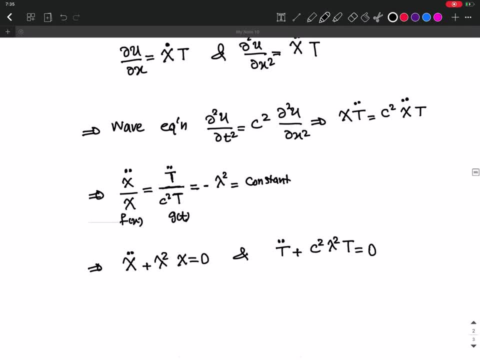 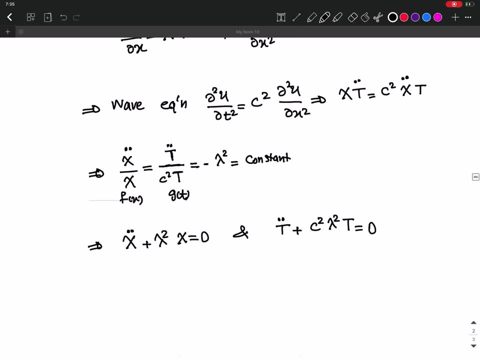 so now i have two sets of equation that i need to solve them separately. i need to solve them separately. i need to solve them separately, okay, okay. so i'm going to start with x. so i'm going to start with x. so i'm going to start with x, so let's get started with x. so the first: 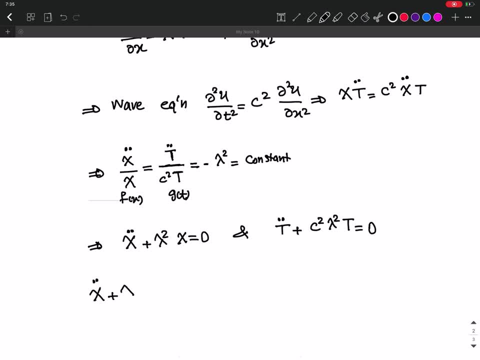 so let's get started with x. so the first. so let's get started with x. so the first equation is x double dot plus lambda equation is x double dot plus lambda equation is x double dot plus lambda square. lambda square x. lambda square x. lambda square x equals to zero. 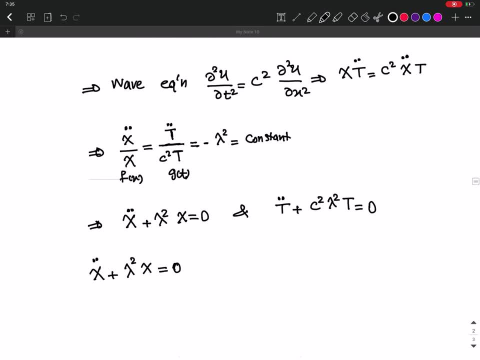 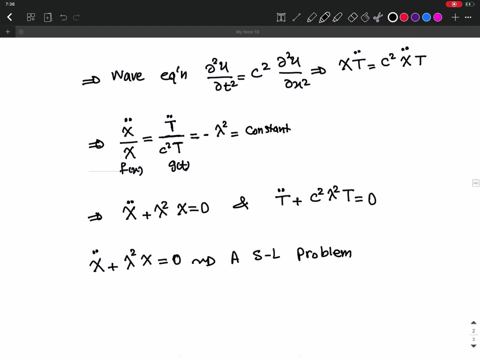 so as you see, so as you see, so as you see, this looks like uh. if you remember a, this looks like uh. if you remember a, this looks like uh. if you remember a storm, leo problem right. storm, leo problem, right storm, leo problem, right. this looks like a storm level problem. 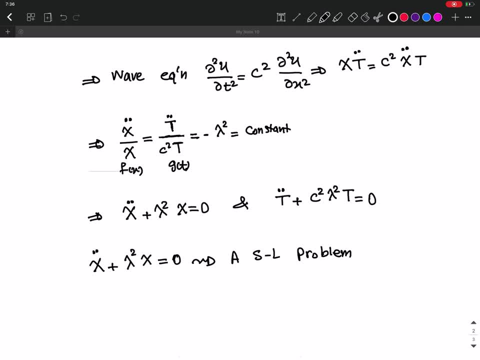 this looks like a storm level problem. this looks like a storm level problem and we know the solutions for this kind and we know the solutions for this kind and we know the solutions for this kind of of of problem. so the solution of this kind of problem, so the solution of this kind of. 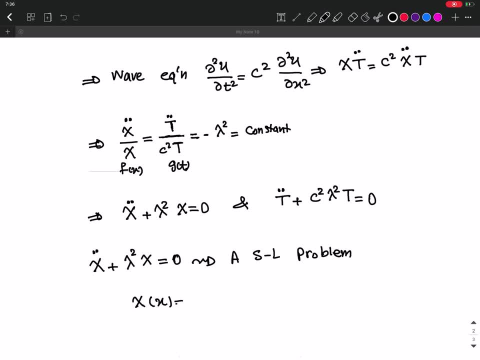 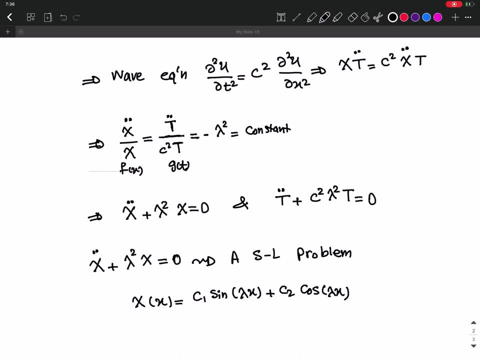 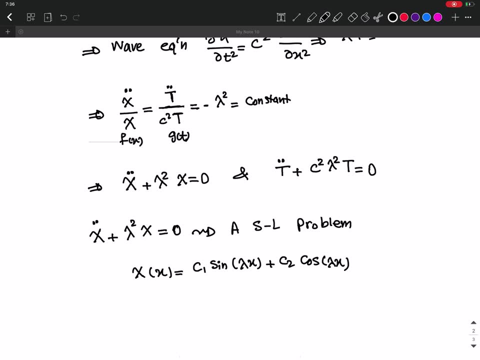 cosine, cosine lambda x. this is a solution from storm level problem. this is a solution from storm level problem. this is a solution from storm level problem that that that we talked before, we talked before, we talked before, and so, in order to find this, c1 and c2. 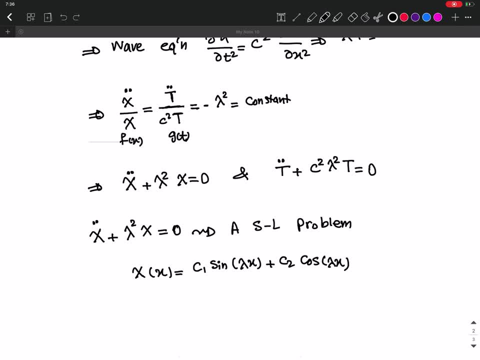 and so, in order to find this c1 and c2, and so, in order to find this c1 and c2, i'm going to apply the boundary, i'm going to apply the boundary, i'm going to apply the boundary. conditions for this problem, okay. conditions for this problem okay. 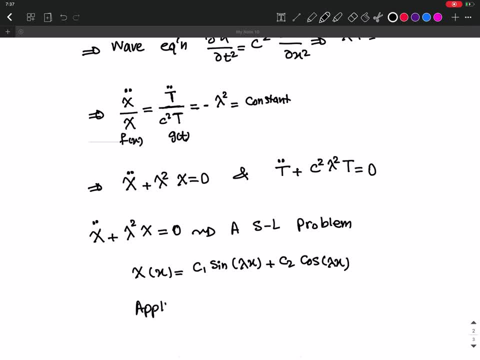 conditions for this problem. okay, so we are going to, so we are going to, so we are going to apply, and this is a general thing. so you apply and this is a general thing. so you apply, and this is a general thing, so you always apply, always apply. 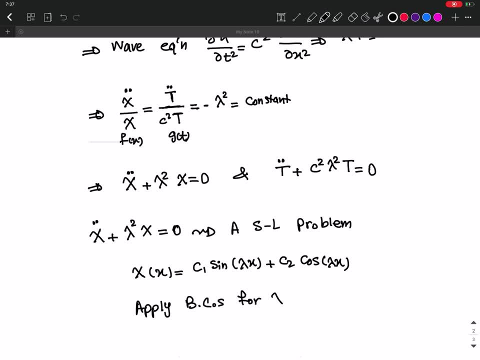 always apply boundary conditions, boundary conditions, boundary conditions for x, for x, for x or the equation of x or the equation of x or the equation of x, and you apply initial conditions for t and you apply initial conditions for t and you apply initial conditions for t. right, because initial condition is. 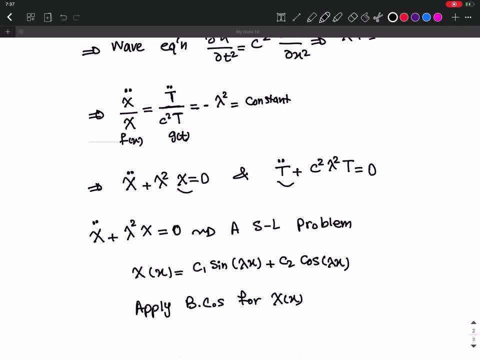 right because initial condition is right, because initial condition is related to time and the boundary related to time and the boundary related to time and the boundary condition is related to space, or x condition is related to space, or x condition is related to space or x. okay, so i'm going to apply boundary. 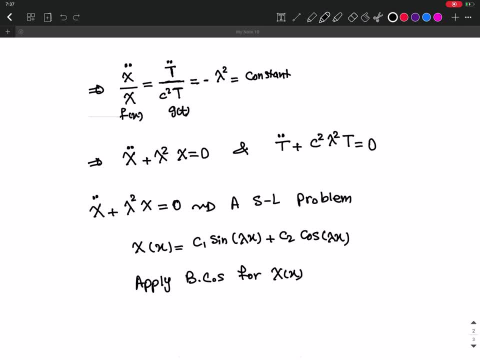 okay, so i'm going to apply boundary. okay, so i'm going to apply boundary: conditions for x in order to find c1, conditions for x in order to find c1, conditions for x in order to find c1 and c2 and c2 and c2. so the first boundary condition is: 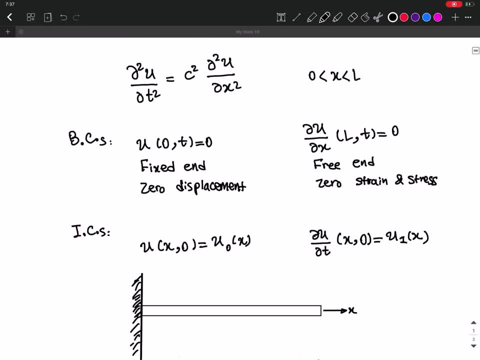 so the first boundary condition is: so the first boundary condition is u at. let's see it here. u at, let's see it here. u at, let's see it here. u at 0 and t equals to 0. u at 0 and t equals to 0. 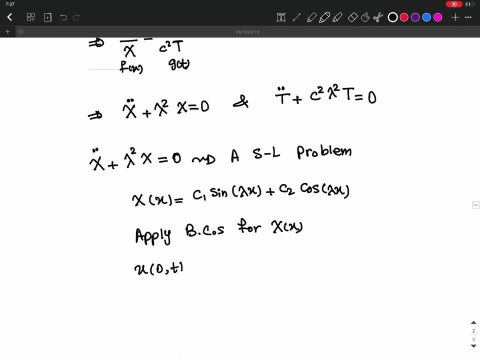 u at 0 and t equals to 0, so so so u at 0 and t equals to 0, u at 0 and t equals to 0. u at 0 and t equals to 0, so this means that x at 0. 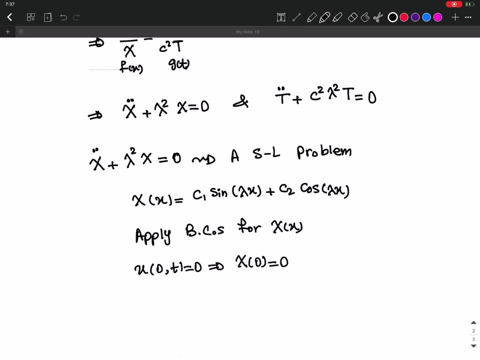 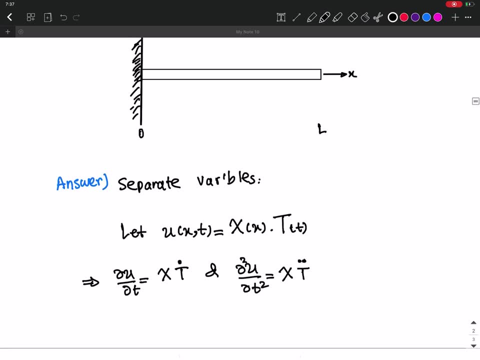 so this means that x at 0, so this means that x at 0 should be zero. and the second boundary condition is: and the second boundary condition is: and the second boundary condition is: what, what, what? partial u, partial u, partial u, with respect, with respect, with respect to. 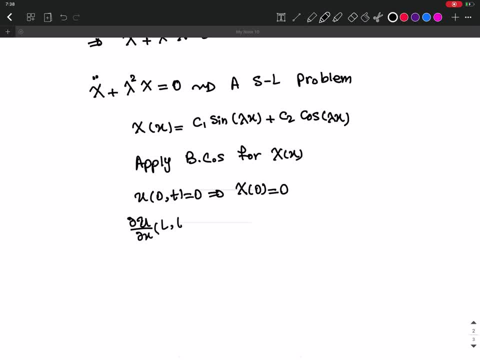 x at x at x at l, and t equals to 0, l and t equals to 0. l and t equals to 0, and this means that x dot and this means that x dot and this means that x dot at l should be zero. okay. 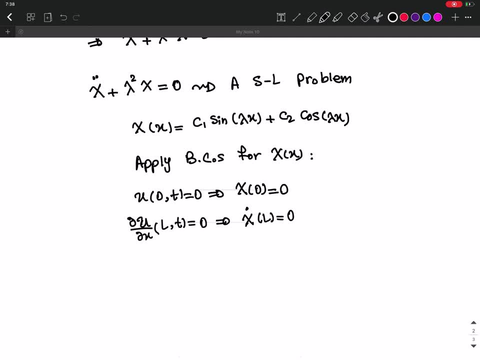 okay, okay, so let's do it for the first one. so let's do it for the first one, so let's do it for the first one. so these are the boundary conditions of, so, these are the boundary conditions of so these are the boundary conditions of the problem. 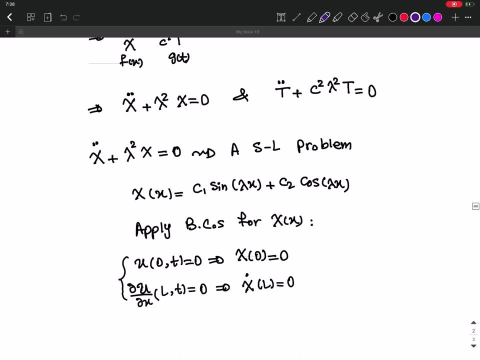 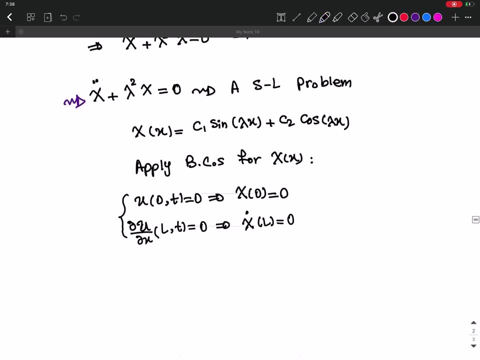 the problem, the problem, and here i try to solve the. and here i try to solve the. and here i try to solve the first equation. okay, so, the boundary condition, and now i. okay, so, the boundary condition, and now i. okay, so, the boundary condition, and now i want to. 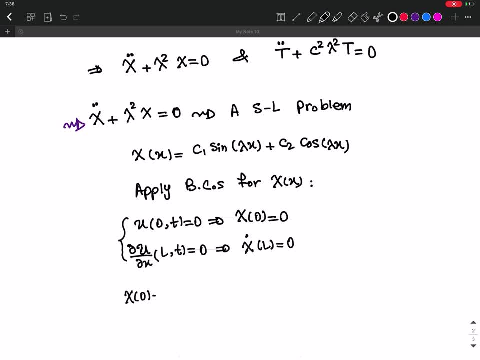 want to want to apply that so x at 0 is apply, that so x at 0 is apply, that so x at 0 is 0. so this means that c1 0, so this means that c1 0, so this means that c1 times. 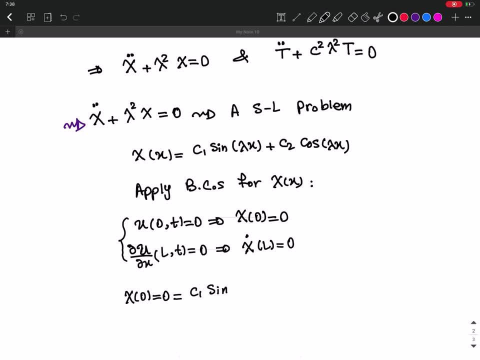 times times sine times sine. lambda x, which is sine, lambda x, which is sine. lambda x, which is sine: 0 plus c2. 0 plus c2. 0 plus c2. cosine 0 is 0 right. cosine 0 is 0 right. cosine 0 is 0 right. so this one is already zero sine of 0 is. 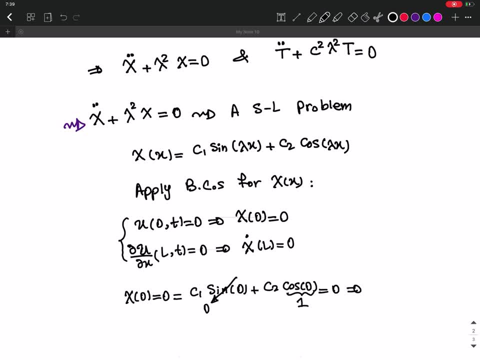 so this one is already zero. sine of 0 is, so this one is already zero. sine of 0 is 0 and this is 1: 0 and this is 1: 0 and this is 1, so this gives me c2, so this gives me c2. 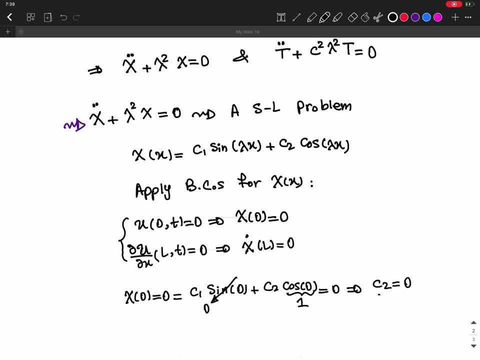 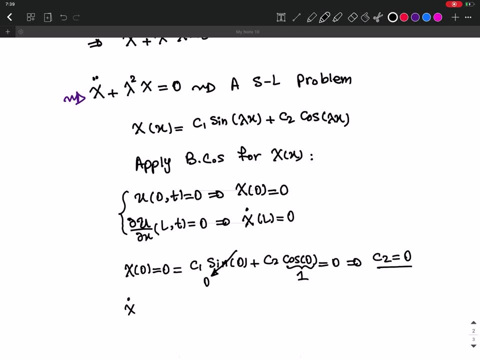 so this gives me c2. is, is, is 0. this is the first result, the. this is the first result, the. this is the first result. the second boundary condition. let's see what second boundary condition. let's see what second boundary condition. let's see what this. 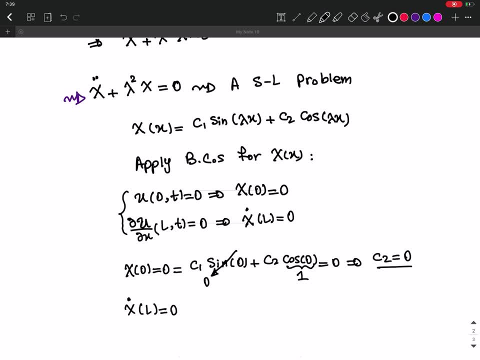 this: this gives us so x dot at l should be 0. gives us so x dot at l should be 0. gives us so x dot at l should be 0, and thus and thus and thus. let's take the derivative. let's take the derivative. 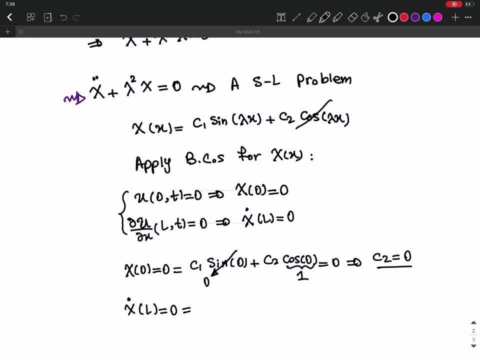 let's take the derivative of x of x of x. so c2 is 0 and we can just take the so c2 is 0 and we can just take the so c2 is 0 and we can just take the derivative of x. derivative of x. 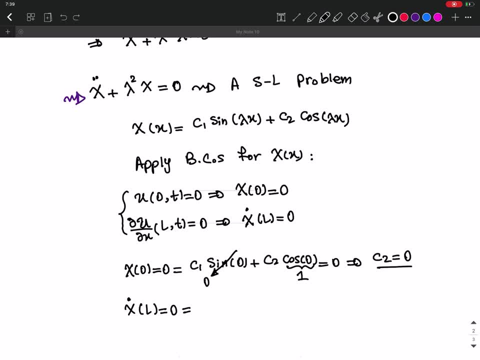 derivative of x of c1. so the first derivative of x of c1. so the first derivative of x of c1. so the first derivative of x is c1 times lambda, is c1 times lambda, is c1 times lambda. cosine, cosine, cosine, lambda. x. right, and instead of x i'm going. 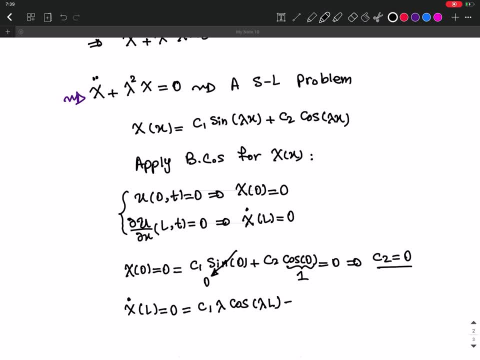 lambda x, right, and instead of x. i'm going lambda x, right and instead of x. i'm going to write l because we are under right to write l, because we are under right to write l, because we are under right. boundary, boundary, boundary, and this equals to zero. 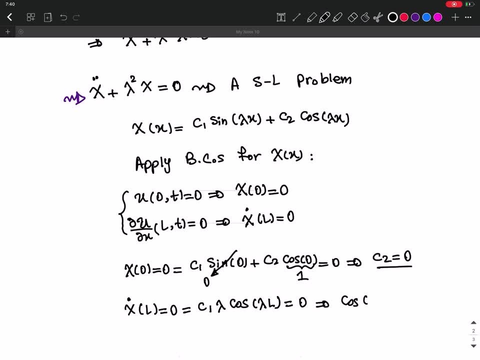 so, so, so, cosine, cosine, cosine, lambda, l, lambda, l lambda, l should be zero in order to not get a should be zero in order to not get a. should be zero in order to not get a trivial solution that c1 is if c1 is also trivial solution that c1 is if c1 is also. 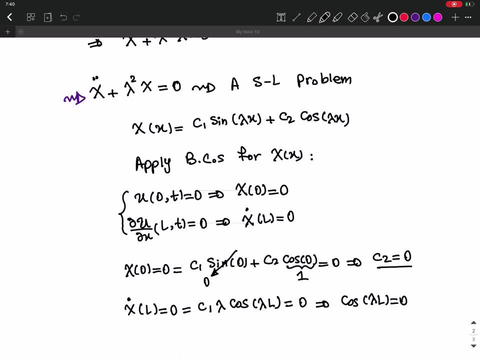 trivial solution that c1 is. if c1 is also zero, then x zero, then x zero, then x is going to be always zero. so we don't is going to be always zero. so we don't is going to be always zero. so we don't want that to. 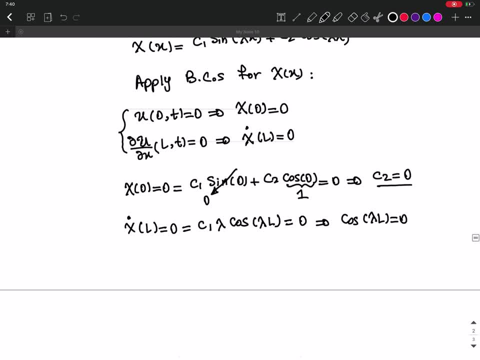 want that to happen. so we can just say: cosine lambda l happen. so we can just say: cosine lambda l happen. so we can just say: cosine lambda l is zero, is zero, is zero. so if cosine lambda l is zero, then we. so if cosine lambda l is zero, then we. 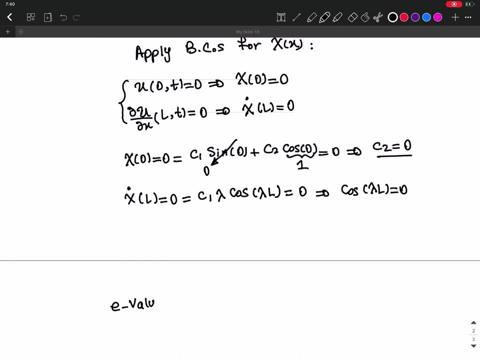 so if cosine lambda l is zero, then we can find the eigenvalues for this, can find the eigenvalues for this, can find the eigenvalues for this problem. that means the solutions in problem. that means the solutions in problem. that means the solutions in which, which, which non-trivial uh, non-trivial, uh, the 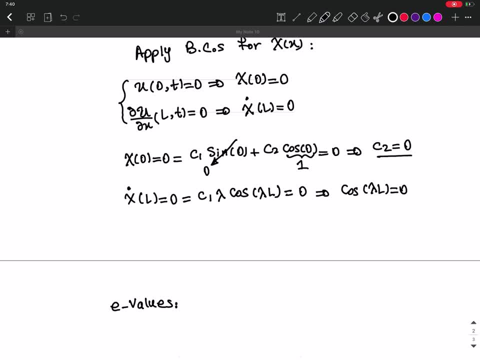 non-trivial uh. non-trivial uh the non-trivial uh. non-trivial uh the lambdas in which lambdas, in which lambdas, in which non-trivial solution exists for this non-trivial solution exists for this non-trivial solution exists for this problem. 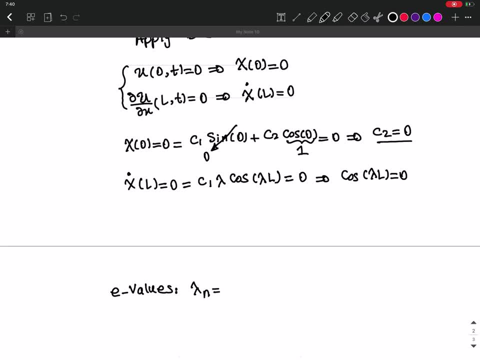 problem. problem is is: is two when? when cosine lambda n, when, when cosine lambda n, when, when cosine lambda n, l is going to be zero. if lambda n is two n minus, let me let me write. it is two n minus, let me let me write. it is two n minus. let me let me write it here, if you. 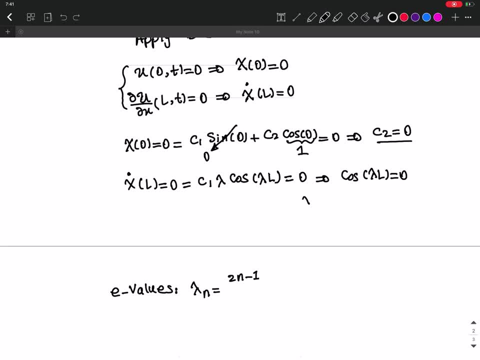 here, if you here, if you don't know so, when cosine is zero, don't know. so. when cosine is zero, don't know. so. when cosine is zero, cosine is zero, for example, for cosine is zero. for example, for cosine is zero. for example, for lambda l equals to 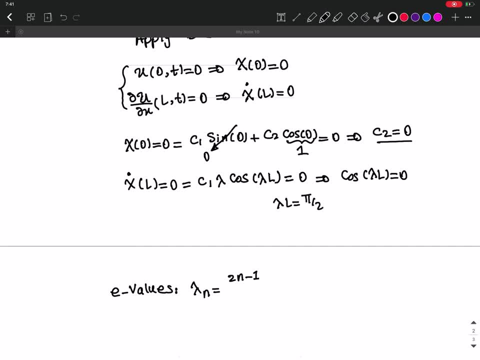 lambda l equals to lambda l equals to pi over two right. this is one pi over two right. this is one pi over two right. this is one, and we're going to do this, and we're going to do this, and we're going to do this, and we can write this as lambda one. 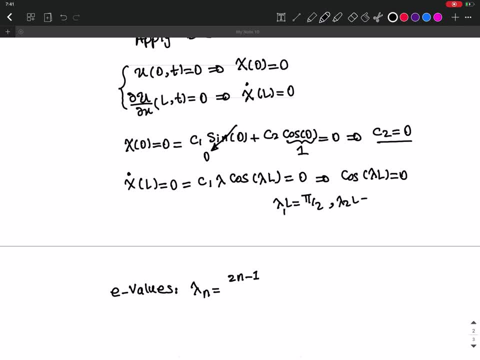 and we can write this as lambda one, and we can write this as lambda one, and then the second one is, and then the second one is, and then the second one is: when it is 3 pi over 2 right, when it is 3 pi over 2 right. 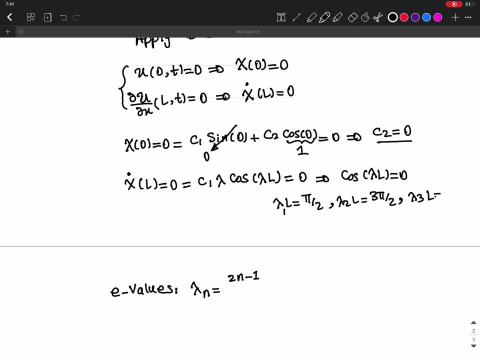 when it is 3 pi over 2 right. and this third one is lambda 3 l and this third one is lambda 3 l and this third one is lambda 3 l equals to 5 pi over 2 right. equals to 5 pi over 2 right. 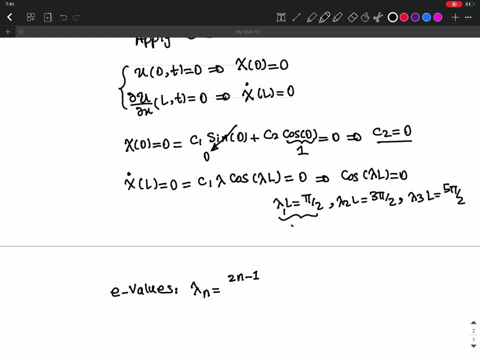 equals to 5 pi over 2, right? so this is going to give me the lambdas. so this is going to give me the lambdas, so this is going to give me the lambdas that i need. so this one is going to say that i need. so this one is going to say: 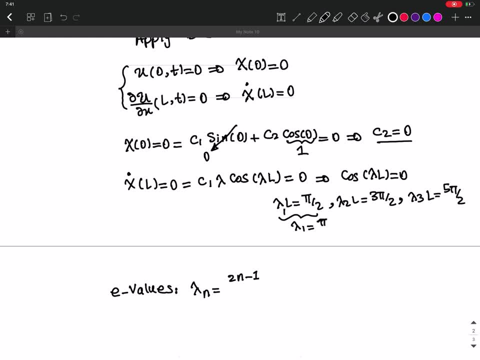 that i need. so this one is going to say: give me lambda 1 is give me lambda 1 is. give me lambda 1 is pi over 2l. the second one is going to pi over 2l. the second one is going to pi over 2l. the second one is going to give me lambda 2 is 3 pi. 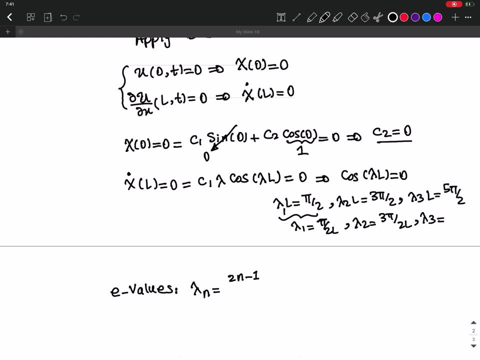 give me lambda 2 is 3 pi. give me lambda 2 is 3 pi over 2l. the third one is going to give me over 2l. the third one is going to give me over 2l. the third one is going to give me lambda 3 is 5 pi over 2l. so 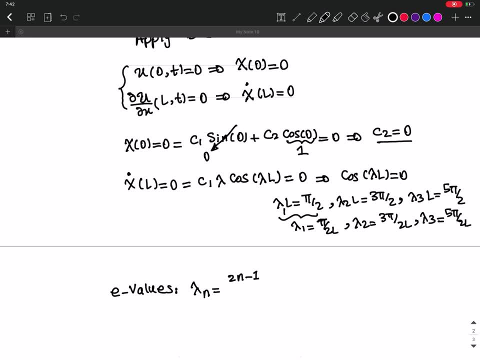 lambda 3 is 5 pi over 2l. so lambda 3 is 5 pi over 2l. so you see the trend here, right? so, uh, this. you see the trend here, right? so, uh, this, you see the trend here, right. so, uh, this is- i'm going to write it as a general- 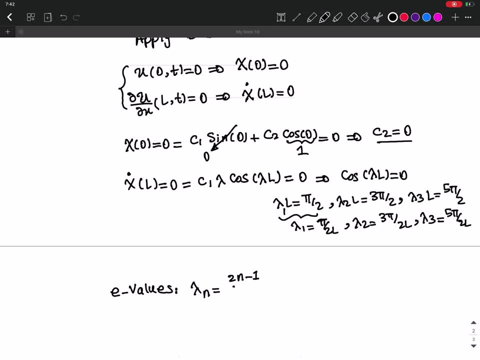 is i'm going to write it as a general? is i'm going to write it as a general formula, as formula, as formula as: 2n minus 1 over 2n minus 1 over 2n minus 1 over 2l times pi. 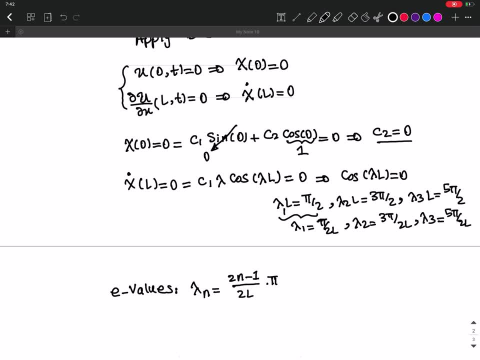 2l times pi, 2l times pi, right, right, right. so this is uh the general formula. and so this is uh the general formula. and so this is uh the general formula. and for, for, for n equals to 1, n equals to 1, n equals to 1, 2. 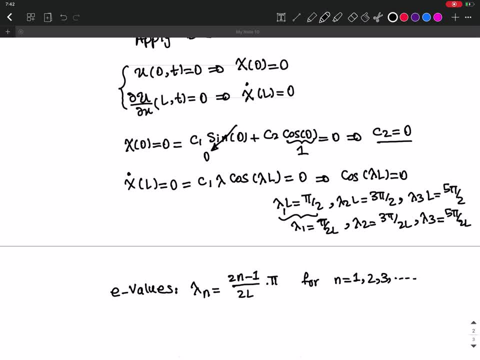 2, 2, 3, etc, 3, etc, 3, etc. right, so i just wrote uh the first three, right, so i just wrote uh the first three, right, so i just wrote uh the first three terms like lambda 1, lambda 2, lambda 3. 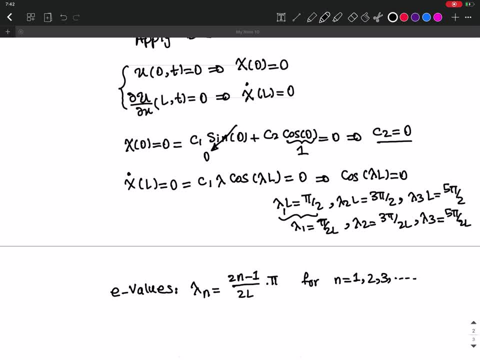 terms like lambda 1, lambda 2, lambda 3, terms like lambda 1, lambda 2, lambda 3 and uh. this follows this formula. so this and uh. this follows this formula. so this and uh. this follows this formula. so this is the general formula. is the general formula. 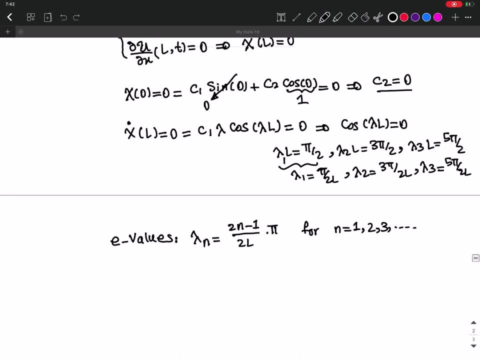 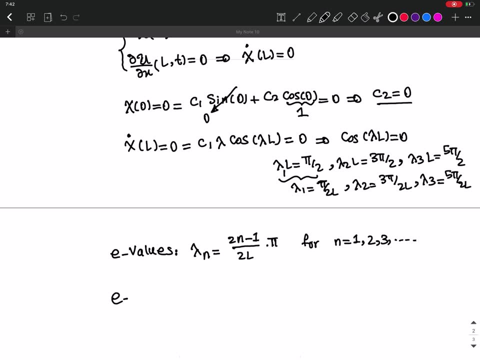 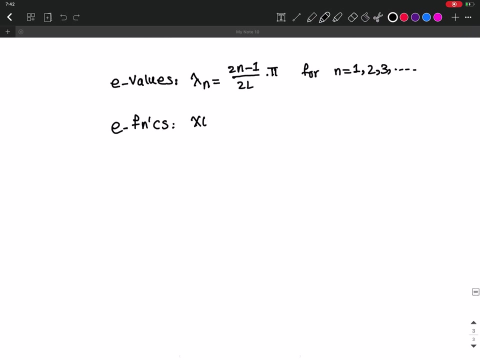 is the general formula: uh for eigenvalues, uh for eigenvalues, uh for eigenvalues, and, and, and, uh the corresponding eigen functions of the corresponding eigen functions, of the corresponding eigen functions of these problem, these problem, these problem are, are, are xx. or let me write it down as: 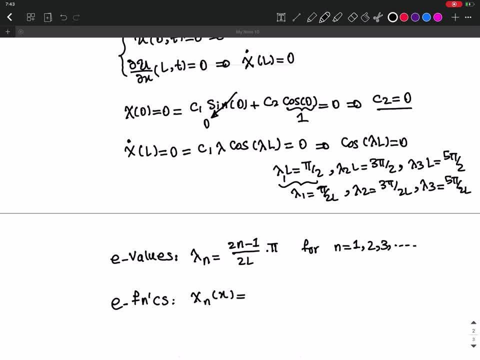 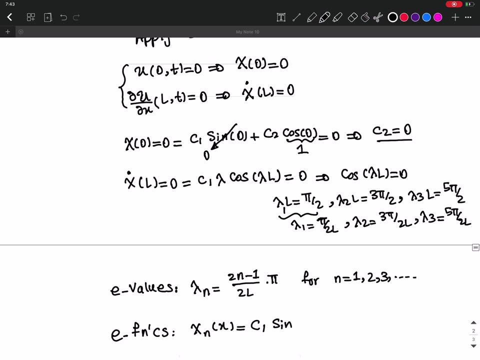 x and x, x and x, x and x, is is, is, is is speech, is speech c1, if you see it here: c1, c1, c1, sin lambda n, sin lambda n, sin lambda n, x right. so these are the x right, so these are the. 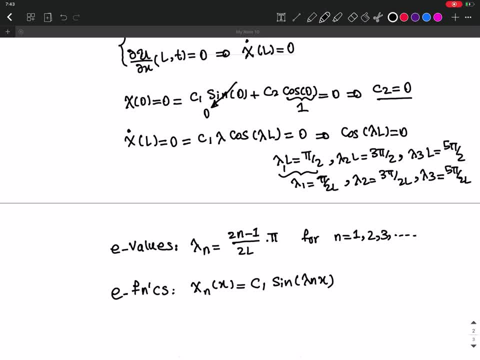 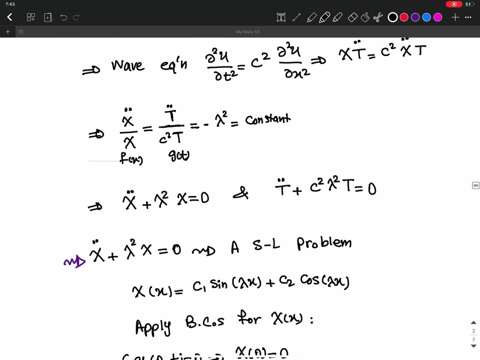 x, right? so these are the corresponding uh, corresponding uh, corresponding uh eigen functions for this problem. Okay, so, before going to the second equation, for time, so this equation, so you already solved this one based on a strong level problem. and then before going to the second equation, 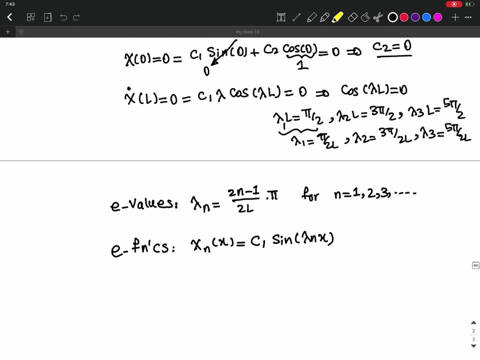 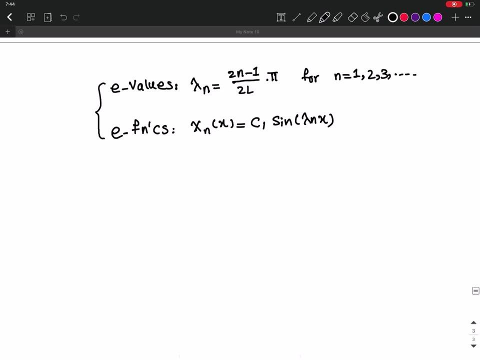 I want to give you some intuition that what, how does this look like and what does this mean? this answer that we found here: eigenvalues and eigenfunctions. So let me show it to you, based on also the boundary conditions that we have here. 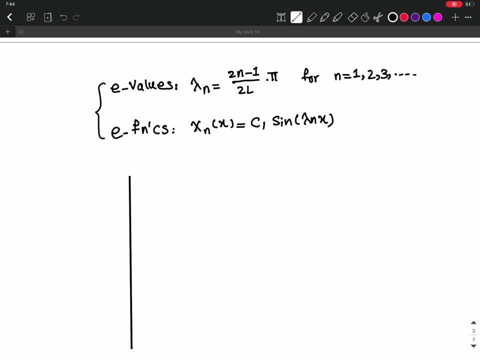 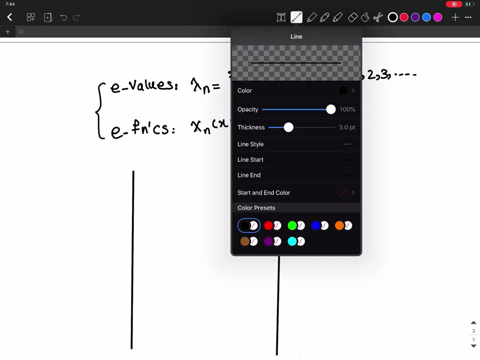 Okay, let me. I want to show the answers of these four, some particular n, So you understand what do these eigenvalues, Eigenfunctions, mean and how do they look like? Okay, so let's say, let me decrease this a little bit and also change the color. 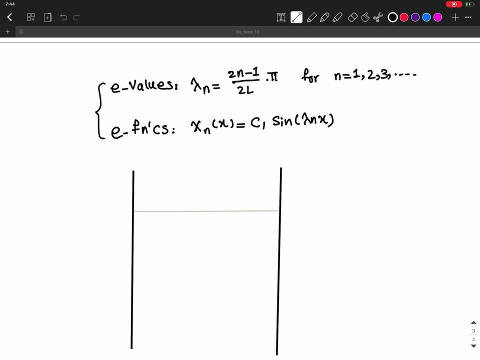 One, two And three- Okay, Okay. so I want to show the solution here: for n equals n- Okay, And n equals n- Okay. So for n equals to 1, for here, n equals to 2, and here n equals to 3, so let's get started. 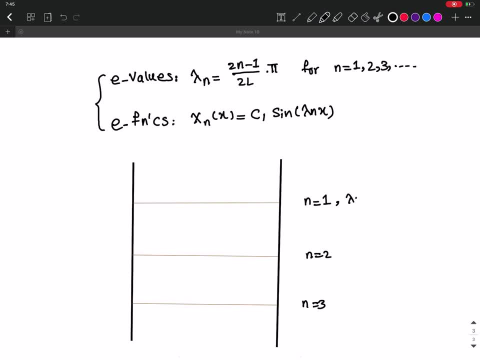 with n equals to 1.. So for n equals to 1, lambda 1 is- you can calculate it from here- pi over 2l and x1, the eigenfunction of this, That is sine pi, x over 2l. 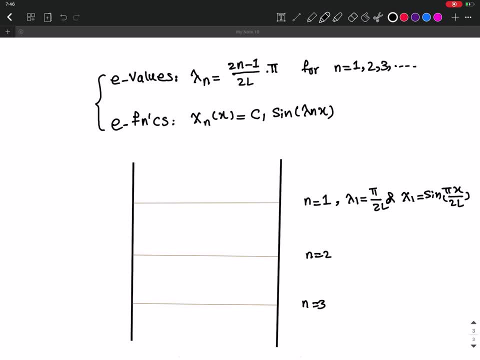 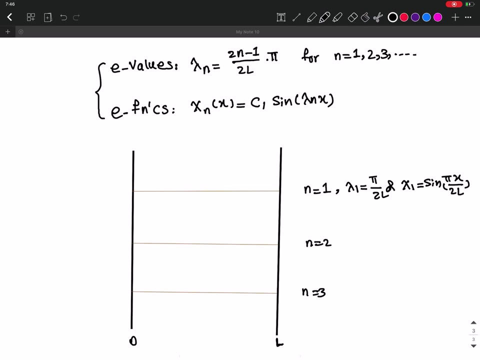 Okay, so if this is 0, and this is l and this is x, this coordinate is x. I want to plot this, So let's plot the first one. So the first one is going to give me something like this: 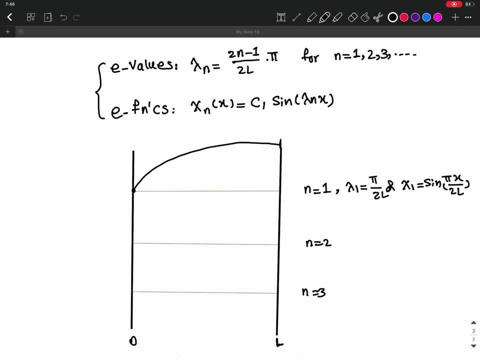 So this is going to give me something like this. So this is going to give me something like this. Okay, So one thing that you notice here that both boundary conditions are satisfied. So x at 0 is 0.. So let me write down the boundary condition. 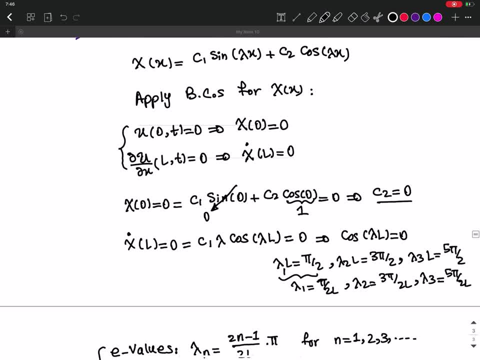 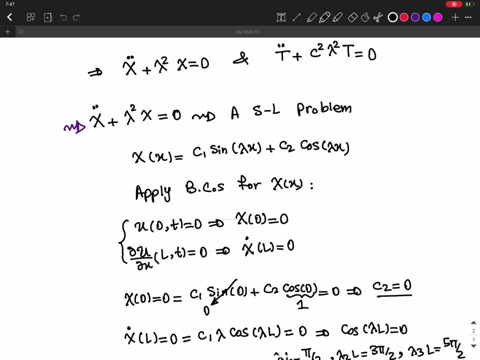 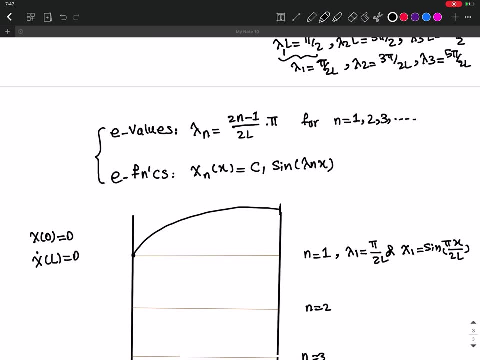 So x0 is 0, right, This is the first boundary condition, This is the second one, And then the second one is x0.. dot at L is 0. okay, so you see, the first boundary condition is satisfied, X: 0 at. 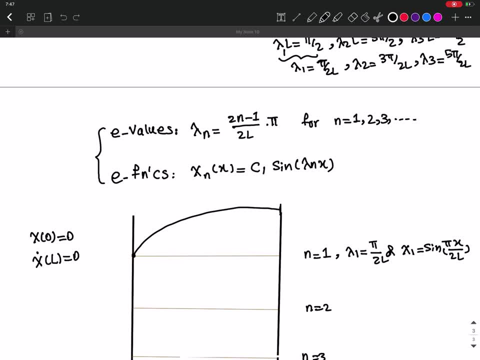 0 is 0 and the second one is X dot. the first derivative of X with respect to X should be 0, and you see it here right. so that derivative is 0. so DX over X, capital X or small x, which is also partial. your partial X is 0 here all. 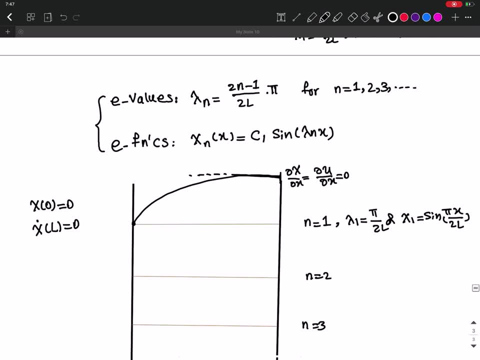 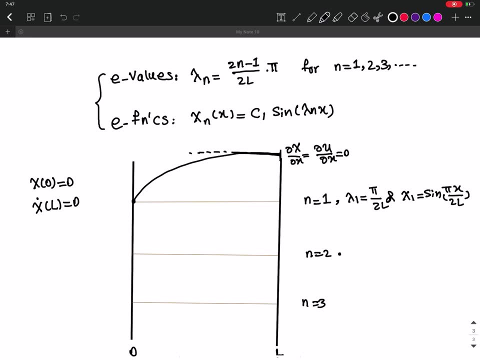 right. so this is the first eigenfunction and the first solution of this problem. so let's go to the second one. so the second one says n equals to 2, so lambda 2 is going to be 3 pi over 2 L and X 2 is going to be sine 3 pi X over 2 L. so 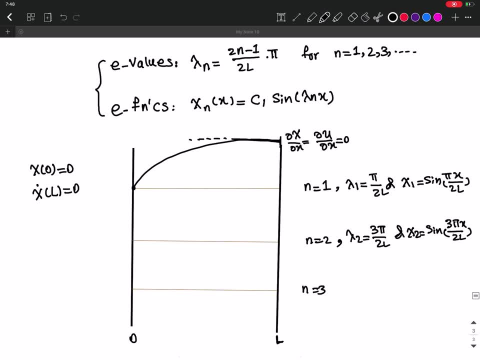 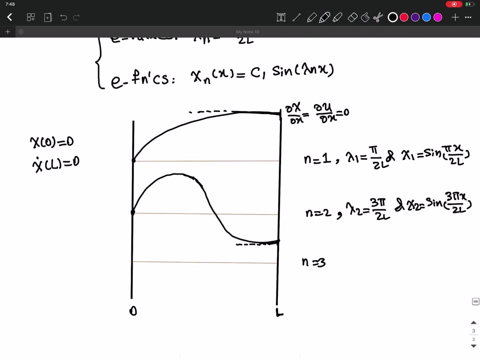 let's see how does this look like. so this one looks like something like this: sine three times per maneuvers, Q would be zero. so, as you see again, the boundary conditions here are satisfied. X at zero is zero, and x dot here is also zero, and this is the second eigenfunction. so X. dot 0 is also consider d Max, and this is the second function. so X dot, huh, and what it device is the second하는 function. so X dot is a state. say I'm sitting here and also taking my graph, that say is ignoring from E4 and myтя mind, and this is the. 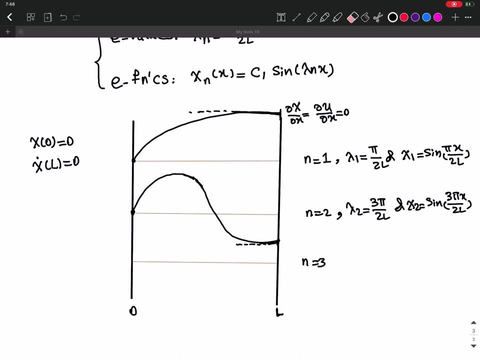 fact that Z plus root equal to zero in the first equation, and for the first 2x, uh, which i showed here, and let me do the third one. so the third one is okay. i don't know why this is not cleaning that. okay, so let me just do it a little bit. 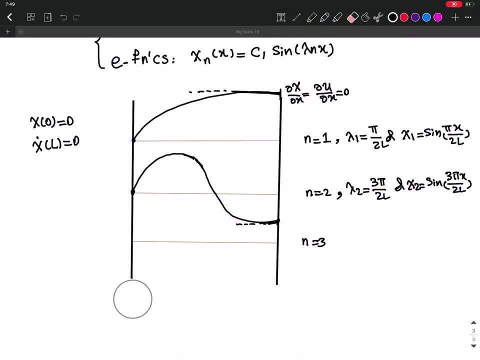 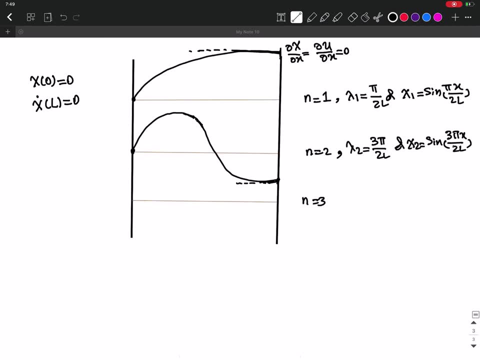 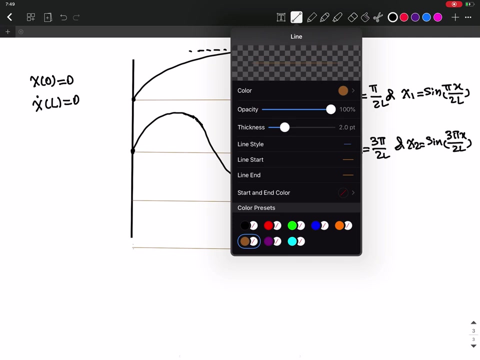 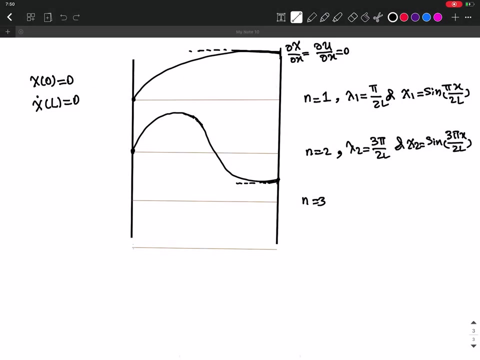 down. so i will plot it here and let me increase this and a little bit more, or i can just do it here like this is easier. okay, so i show n equals to 3 here, so n equals to 3, then lambda 3 is gonna be 5 pi over 2L. 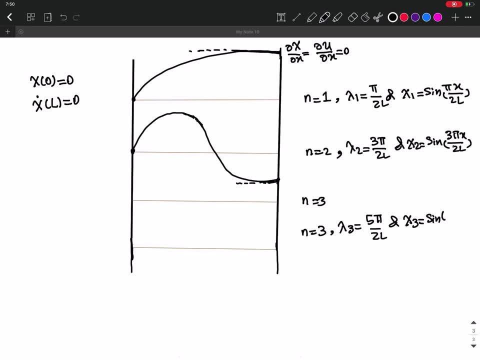 and x3 is gonna be sin 5 pi x over 2L. okay, so let's draw this one. so this one draw, we get something like this. so we are gonna do this. yeah, try to dry it. well, yeah, something like this. okay, let me clean this a little bit. 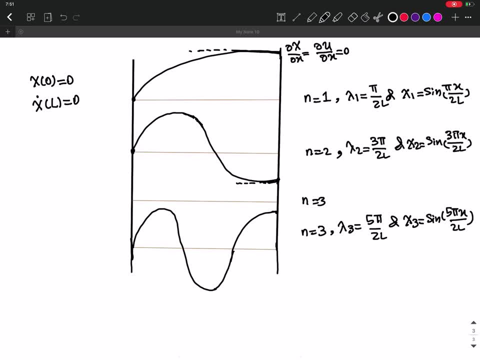 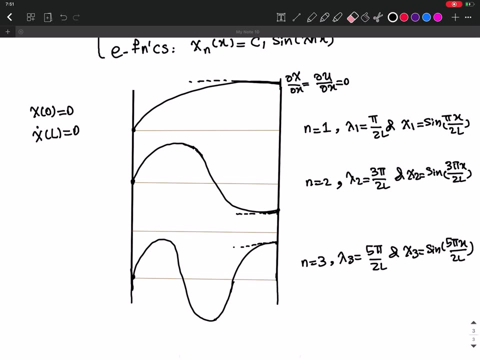 so you see, now also, both boundary conditions are satisfied here. so we have these three mode modes and, uh, you see, these are just the first three, and this can go and on and on, okay, up to up to infinity. so, uh, this can go on and on up to. 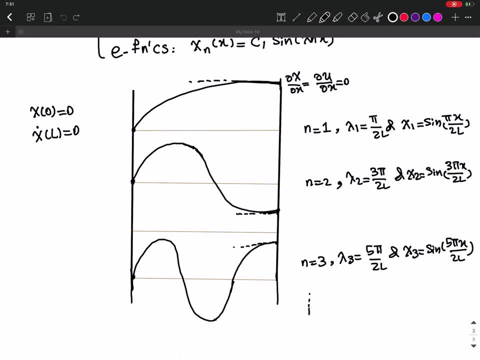 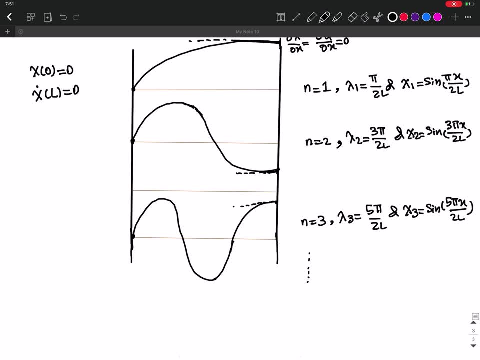 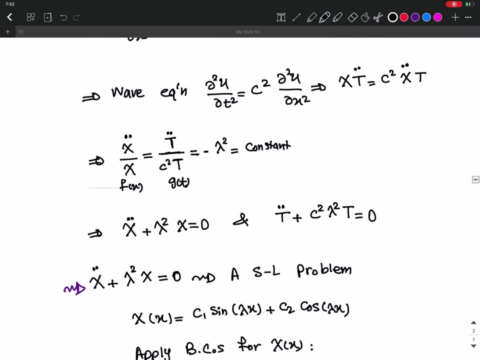 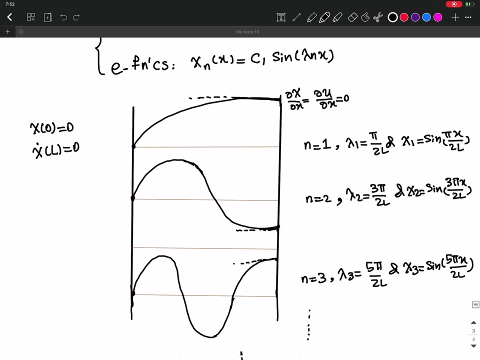 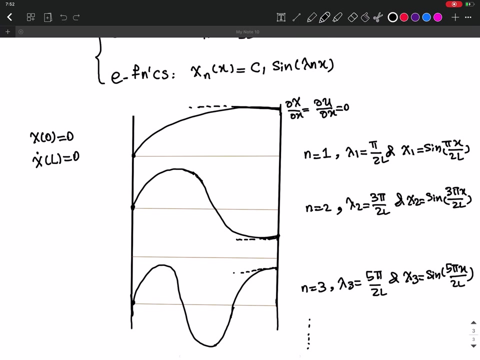 okay, infinity and infinity, and these are, as you see, called. so these are called modes of vibration. so these are modes of vibration. so when you're being vibrates, these are the functions that vibrate. so, for example, if you say mode one of vibration, this means the first mode, is this one right? and then if you say the second mode, this is going to be. 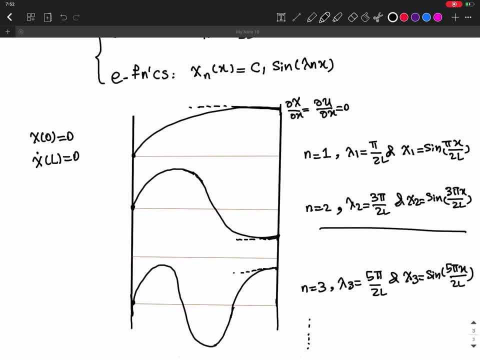 the second mode and the shape of it is, uh, shown here, the second mode of vibration. and finally, if this is third mode, this, this, this is going to look, this is the third mode, right, and then you can go on and on. so uh, for example, sometimes you can say, like the first modes are. 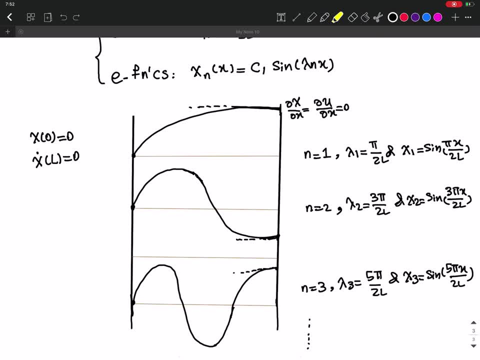 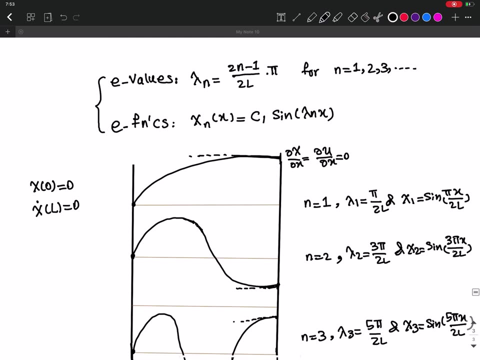 stronger, or then, uh, the strength of the higher modes is uh like weaker. something like this depends on your problem. so these are actually what we call the modes of vibration. okay, and this is how your, for example, um beam, uh displaces of vibration, and this was just to give you uh intuition that. how do these solutions look like the